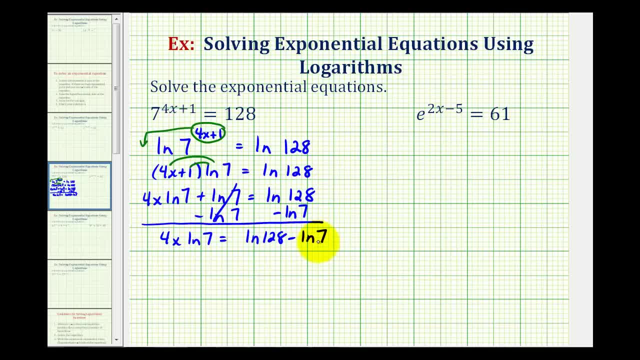 Remember we cannot subtract these because these are not like logarithms. And now to solve for x, we need to divide. so we'll divide by 4. natural log 7 on both sides. Notice on the left side: 4 over 4 simplifies to 1.. 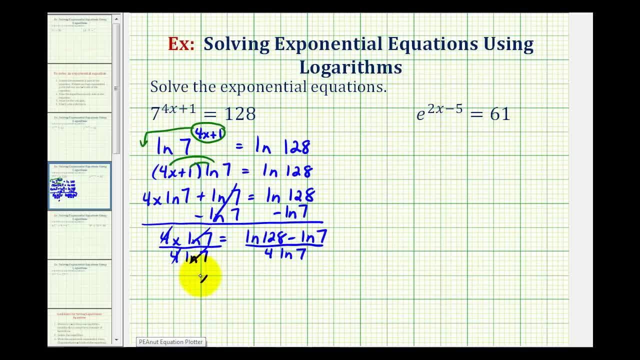 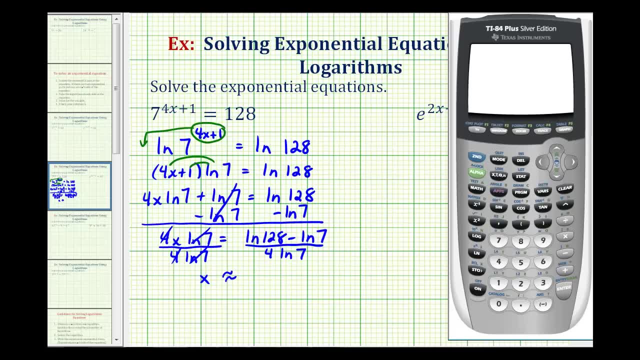 Natural log 7 over. natural log 7 simplifies to 1.. So we have: x equals this quotient. but now we'll have to use the calculator to get a decimal approximation. So we'll have a set of parentheses around the numerator and the denominator. 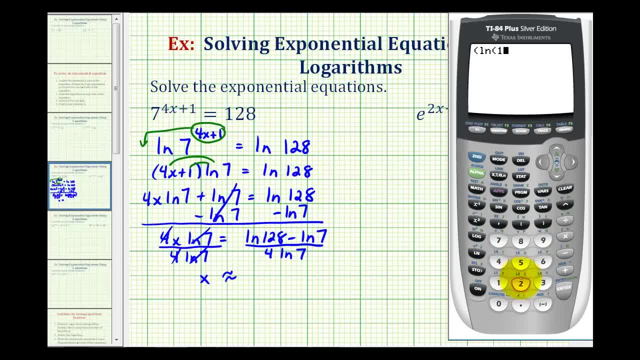 So we'll have an open parenthesis: natural log 128 minus natural log 7.. So there's the numerator divided by our denominator of 4, natural log 7.. And it's typical to round to four decimal places. so x is approximately 0.3734.. 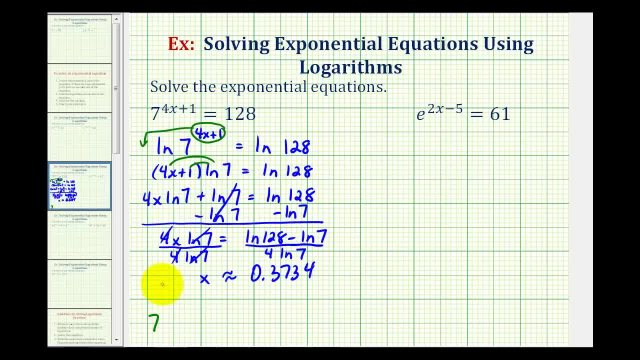 And to check this, we want to raise 7 to the power of 4 times 0.3734 plus 1. And this should be approximately equal to 128.. Let's go ahead and check to make sure that our solution here is correct. 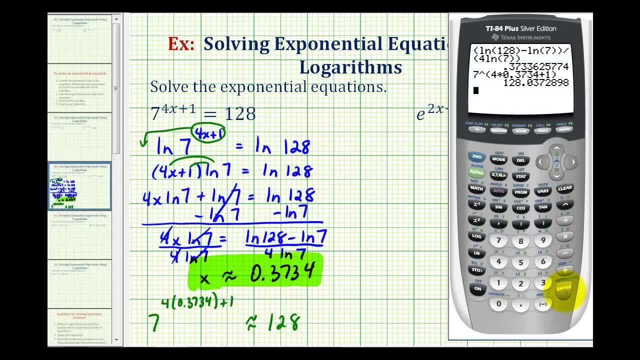 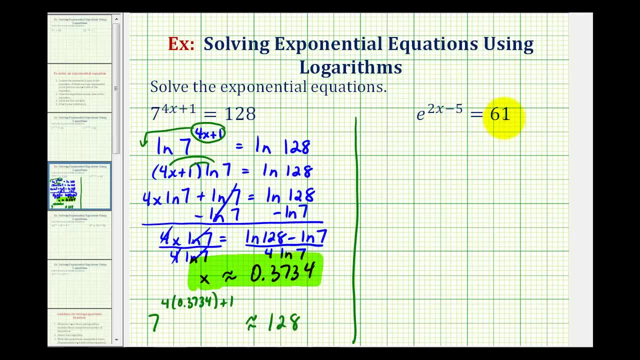 And we did round up slightly. therefore, the value is a little bit larger than 128, but this does verify our solution. Let's take a look at another example. Here we have e raised to the power of 2x minus 5 equals 61.. 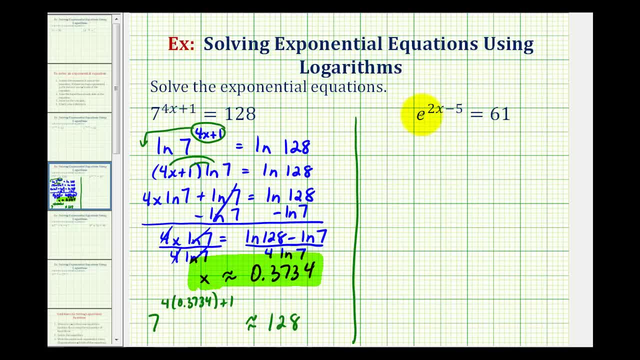 Again, the exponential part is already isolated. But since here we have base e, it's going to be easier if we use the natural log rather than the common log. So if we take the natural log of both sides of the equation we would have natural log of e raised to the power of 2x minus 5. 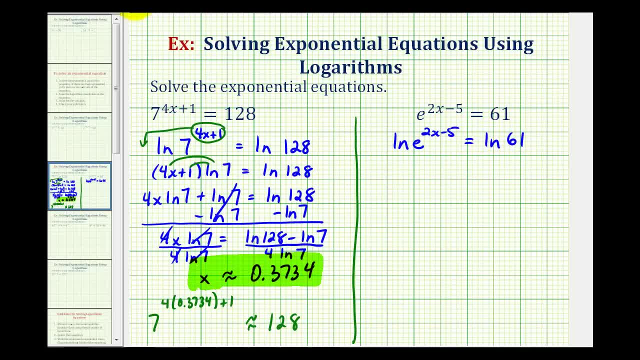 equals natural log 61.. And again we can move x out of the position of the exponent by applying the power property of logarithms. So we'll move this to the front. So now we have the quantity 2x minus 5 times natural log. e equals natural log 61..